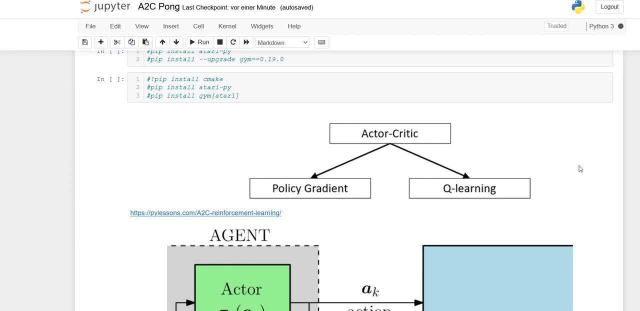 To just recap what we were doing last time: we already implemented the actor critic model who was used with the environment of the Acrobat, So we were choosing the Acrobat. you can also use the pendulum and so on, So there are a lot of interesting environments actually, and this time we are going to use Pong for the required environment. 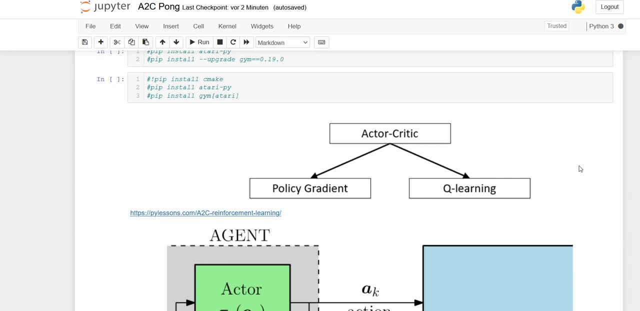 So to just recap what we were doing last time as well as what we are going to do today. So, basically, what is actor critic? So you have on the left side the policy gradient and the queue. So two methods are going to be fit together into one model and one approach. 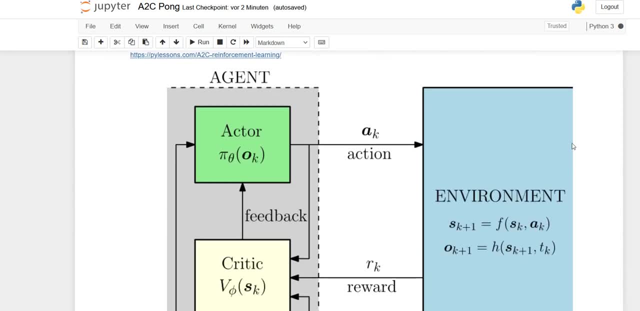 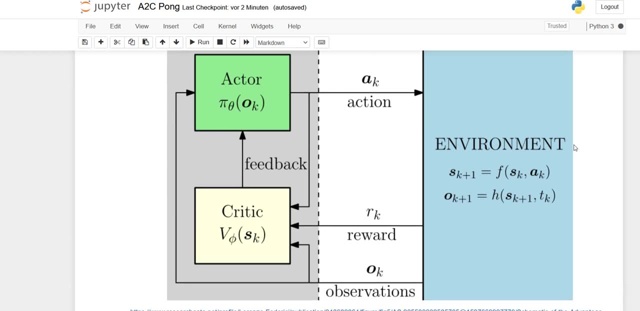 So basically, if you put them both together, you can see that the actor is the on policy model and the critic is the off policy model, So the value based model which you know from queue learning. actually Queue learning is an off policy model and the actor is the policy model, so the on policy model in this case. 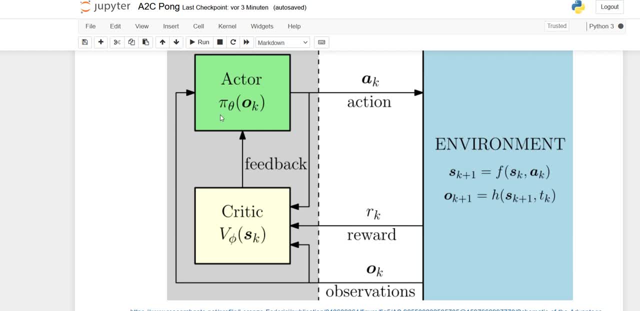 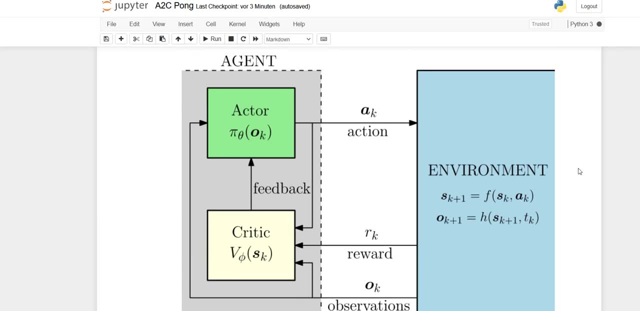 That's why you can see the phi, which stands for a policy. So the actor critic. actually, what they are doing is that you have the actor who gets as an input the actions, The states. So within the states, the neural network is deciding the proper action right. 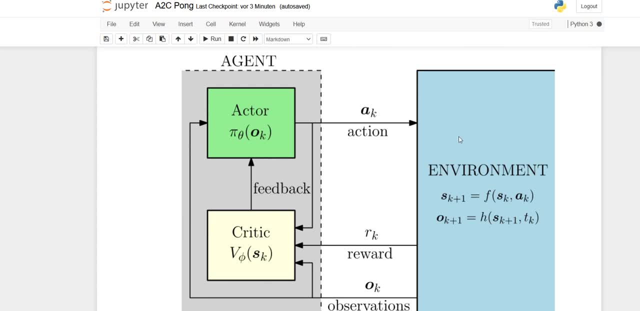 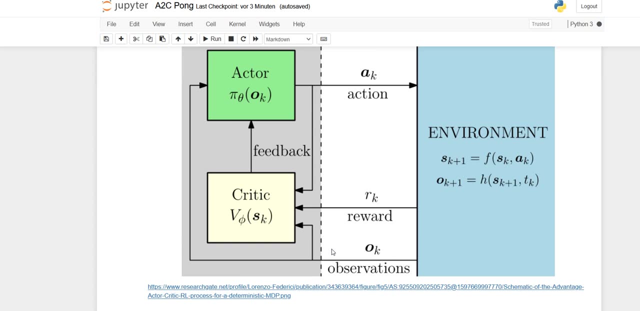 So you can see the arrow here going to the right, to the environment, The environment itself- it's delivering the observations- or the state itself, where the states are going to the actor, because he has to adjust the observations And the actor is actually calculating the best. 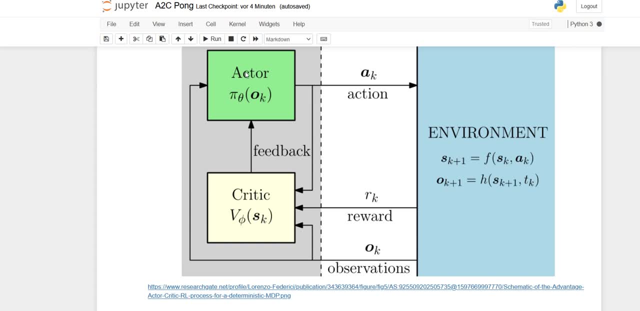 Or determining the best actions, And based on this, he's receiving some feedback from the critic, And this is something similar to GANs, So to general advertising networks, Generative advertising networks, something like this. So you have kind of two models. 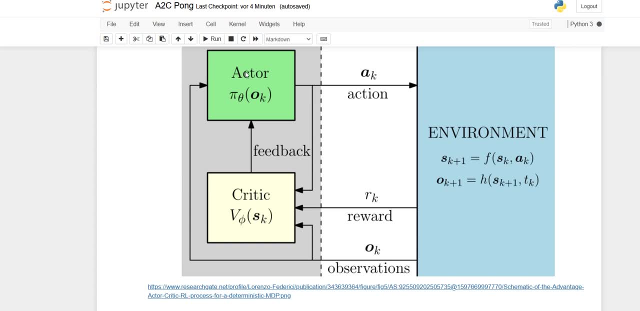 The one is doing something calculating, determining the action, And the critic is giving him some tips how to receive a higher, let's say a higher Q value or a higher reward, by doing so to determine the best action here or the max reward. 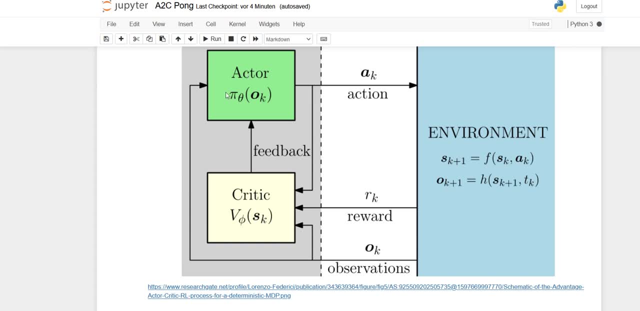 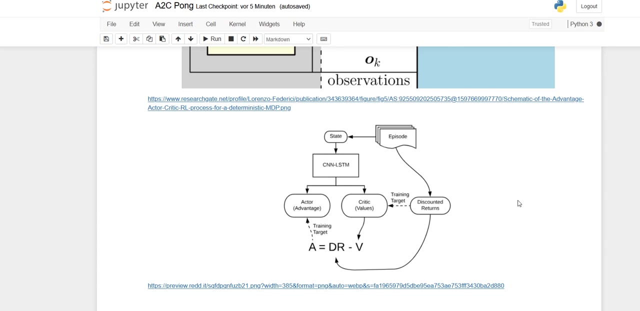 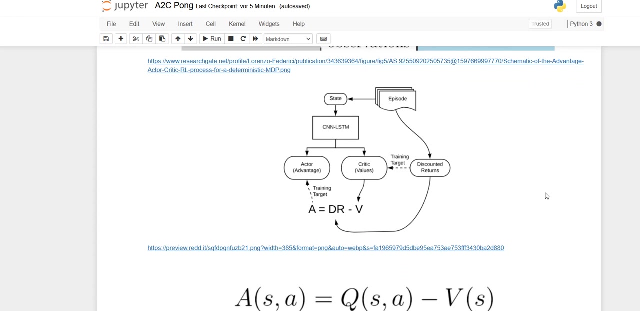 So through the environment here The reward is also passing to the critic And as well as the observation is also passed to the critics. So they're kind of a team in this phase. actually, To just see why this time, Because last time we were covering the topic actor critics. 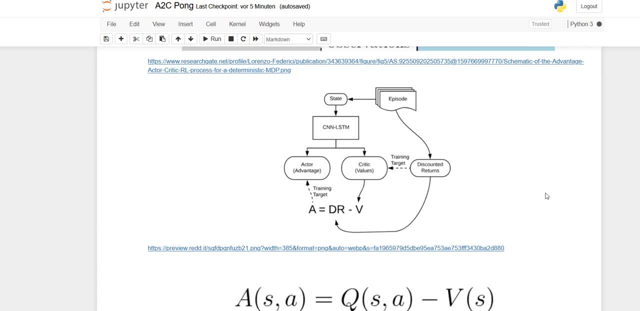 We set up a model because they're playing like a really proper and good team. So everybody of them is getting better and better through time, through episodes And how they're doing it. actually You can see that in this kind of continuous environment here. 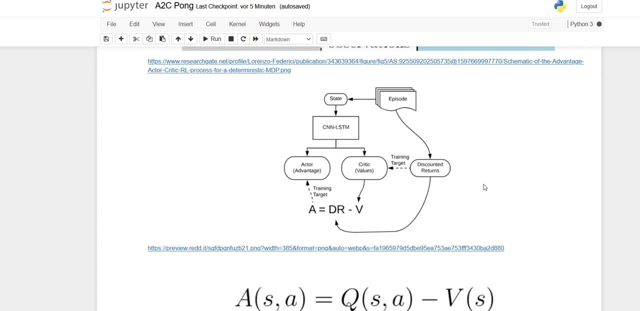 Where we have CNN LSTM, Who is actually taking the input environment and passing them to the actor and the critic. So the actor there, Who is calculating The advantage, Gets the discount return on the right side from each episode And this discounted return is. 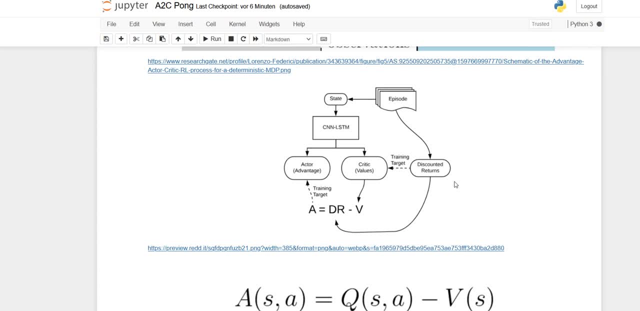 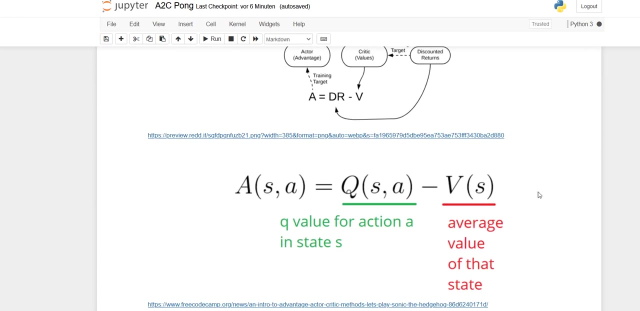 You have to This minus the value If you subtract both of them. So you take the value from the critic actually, And then you receive the actual actors advantage, Which is what it's all about, As you can see here in this formula. 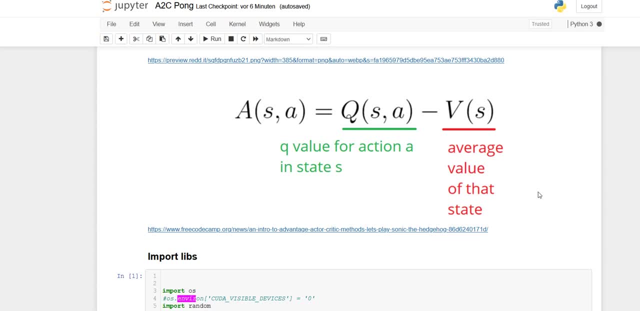 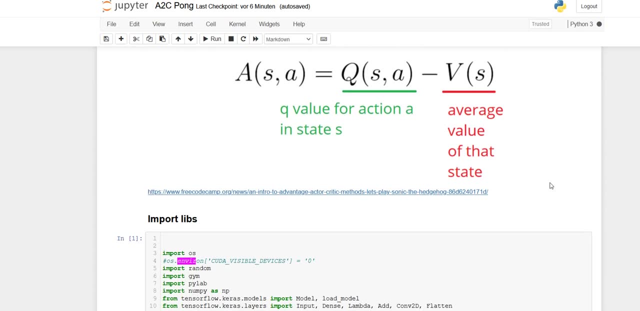 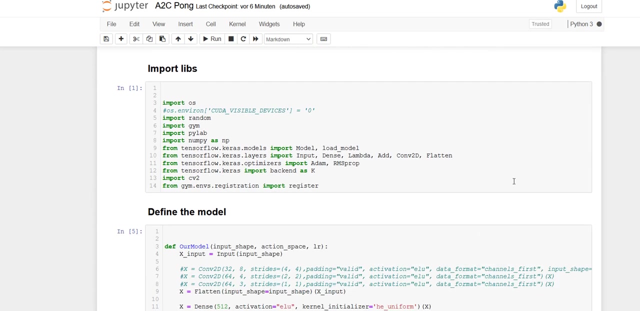 You got the Q value from the action in the state And you subtract everything with the average value of the state To receive the advantage. So To Start with all the topic, First of all, How we are going to implement this in Python. 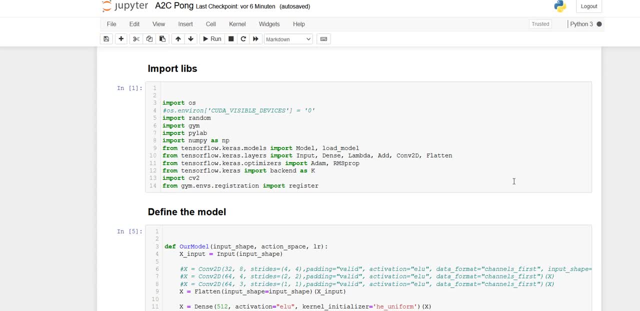 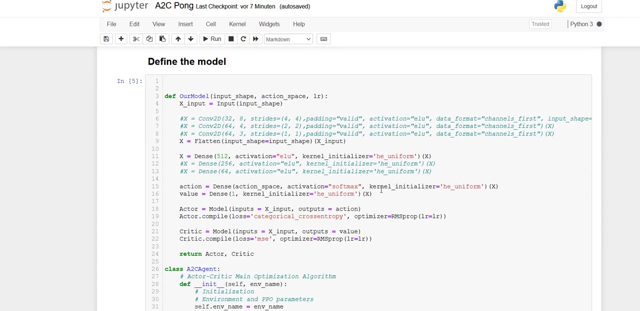 So basically I'm importing the libraries here, Like TensorFlow Gym And PyLab and so on. So Then afterwards I'm going to define the model right, Because We have the actor and the Critic model here, as you can see. 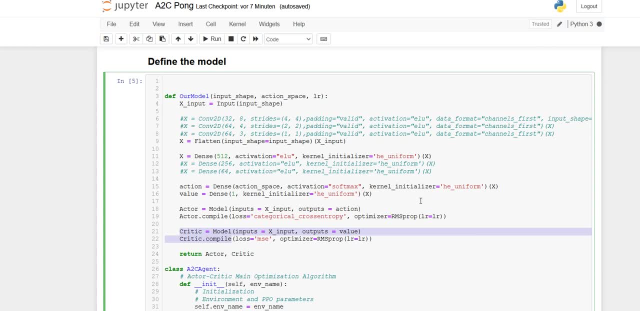 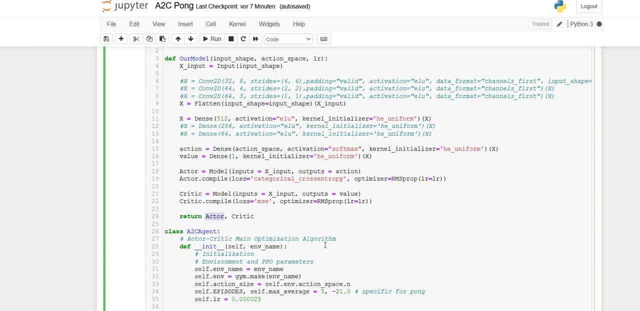 And They are returning the This Yeah Constructor here, The actor and critic one, And There are just basically two networks Who are passing All the return value from this. So the actor is passing the action And the critic is passing the. 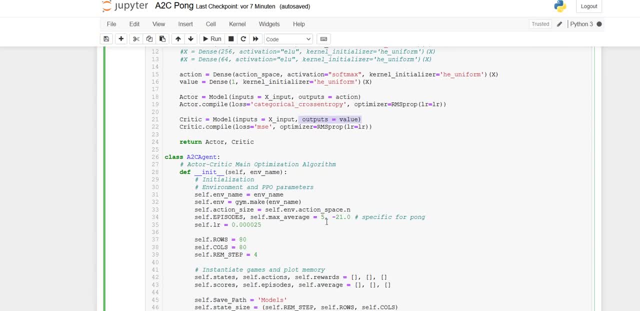 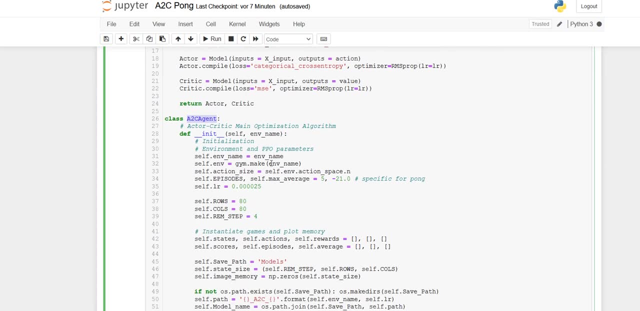 Value here, as you can see from the output. So by starting the A to C agent From this Constructor here, You are setting the parameters Like Episodes, So I'm basically just taking five. So Because I don't have a GPU, 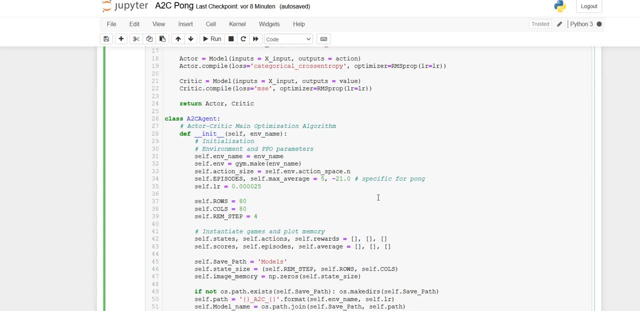 Set up here on this Laptop, So I'm just using five To just demonstrate everything. But if you have a GPU, Just Insert, For instance, Hundred Episodes To just get started, To have a really nice Result. 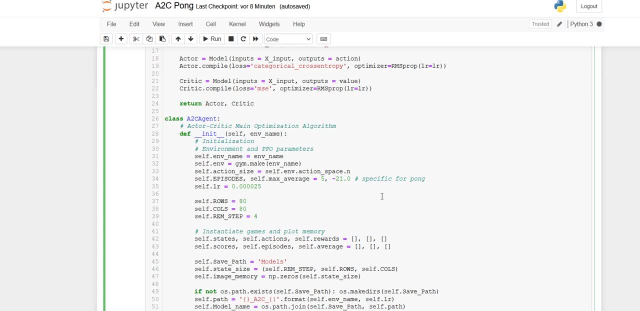 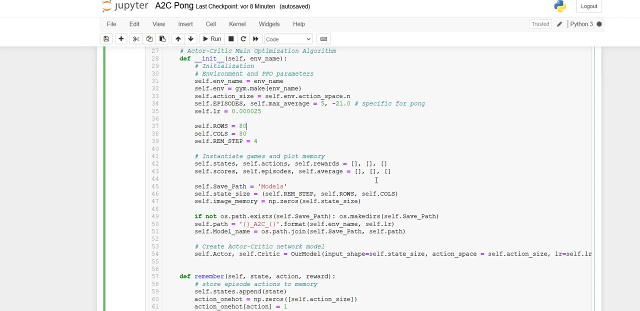 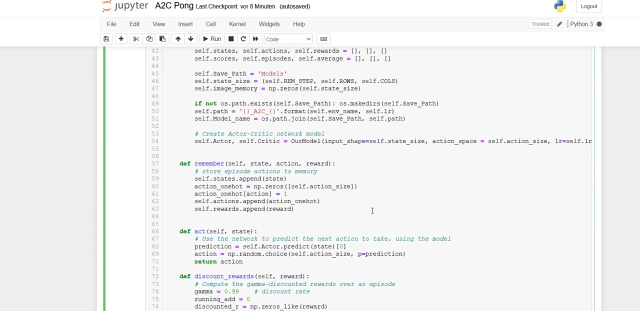 So I'm just Using Five To just Demonstrate Everything, And After this You can basically Go further To Store All the episodes And actions To memory. This Method Here That you can see: 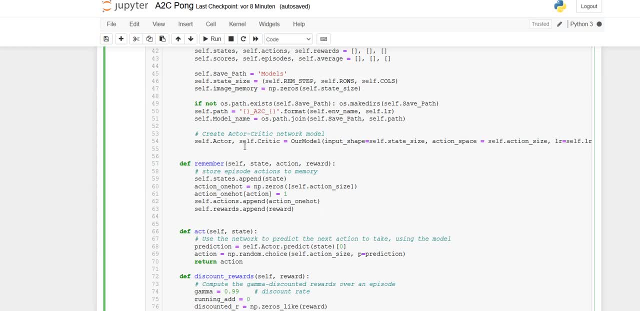 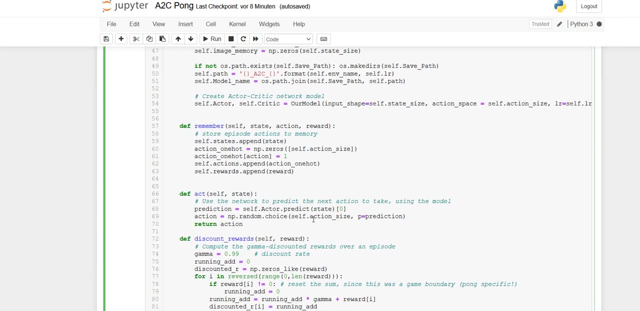 Define, Remember And All the actions And rewards Are going to Be stored. After this, You're going to Use The network To predict The next Action, So This Is The next Action. 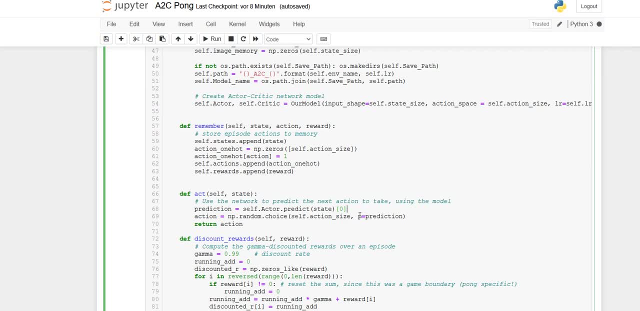 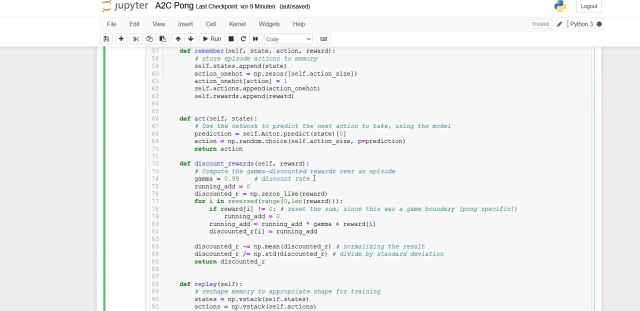 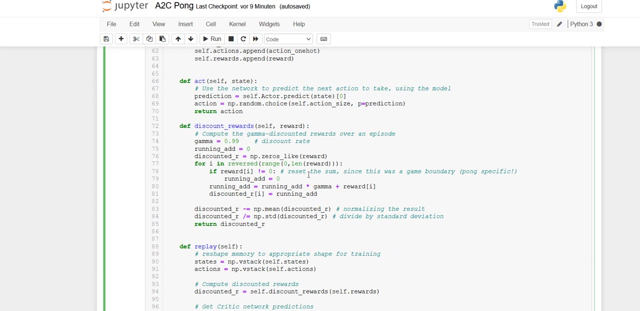 Using The model, So You're Basically Predicting Everything With The Actor And Taking The Random Choice As An Action. After This, You Have The Discount. 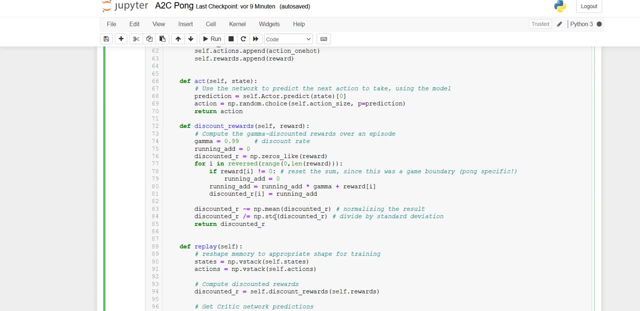 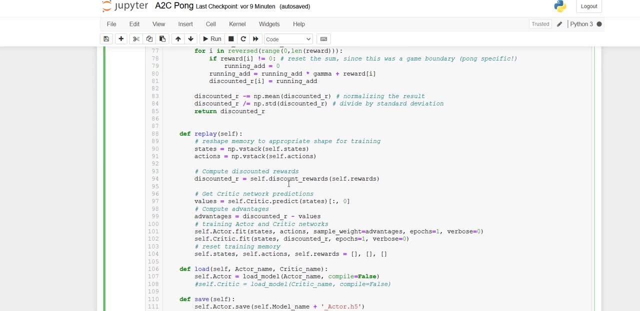 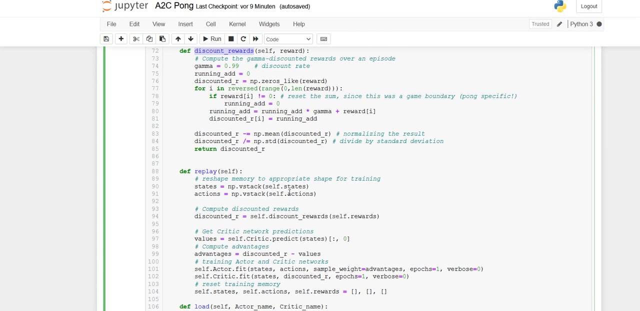 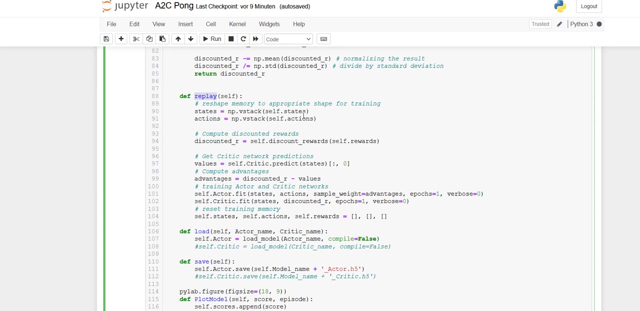 Reward This Then As You Can. So In The Formula We Have The Discount Rate Here. So This Was This Discount Reward. Who Is Going To? 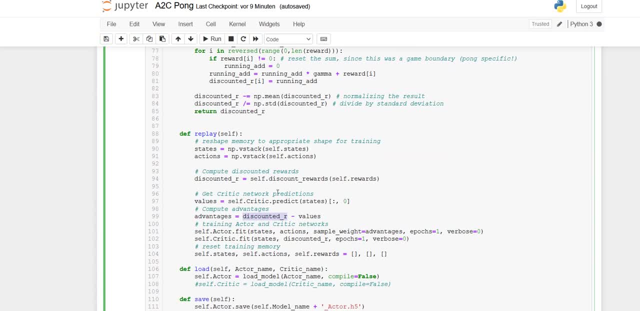 Be Calculated And In The Discount Rate Which Is Consigned And Picture Bow Is Going To Be Substracted With The Value That You Can. 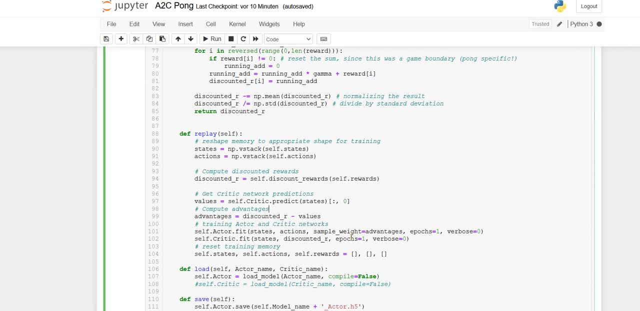 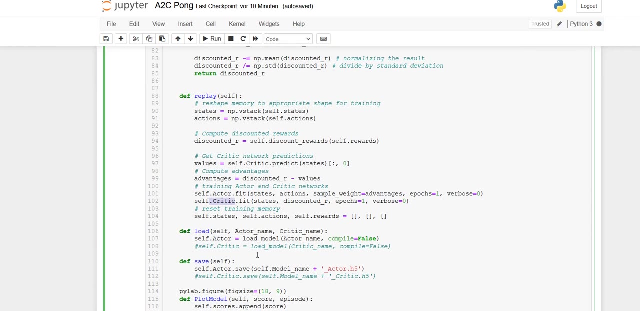 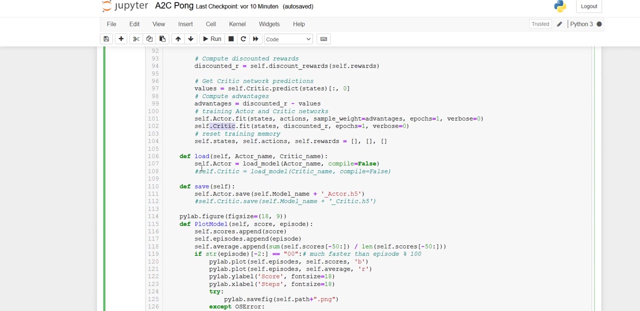 Get From The Critic Discount Rate. You Can Get From The Discount And Is Going To Be Training The Actor As Well As The Critics. 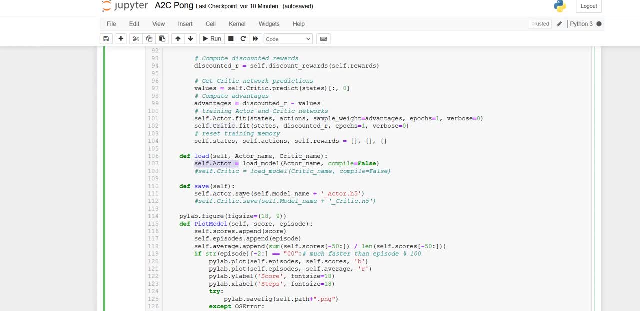 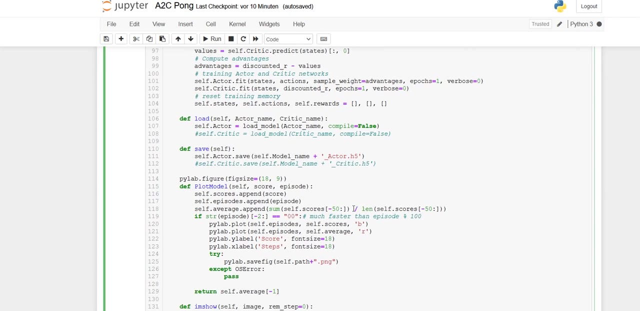 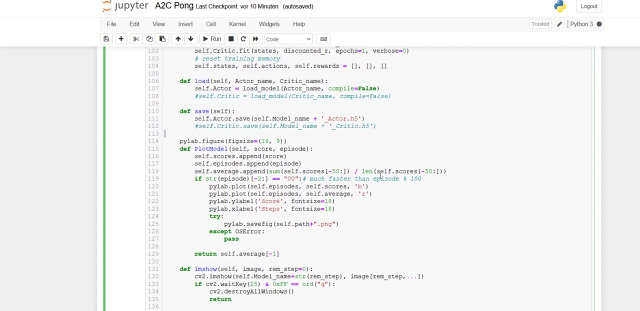 And Yeah, Then You Are Calculating The Actions, The Rewards, And So Afterwards You Want To Save Everything Right, To Reuse It, To Plot The 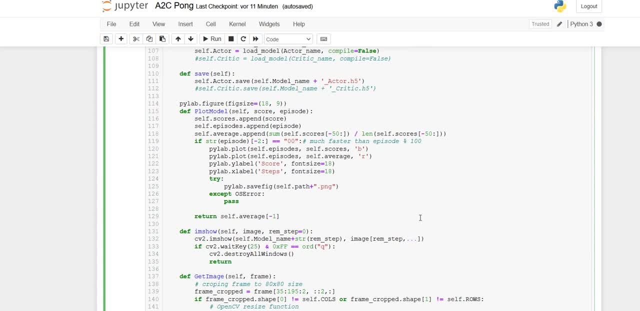 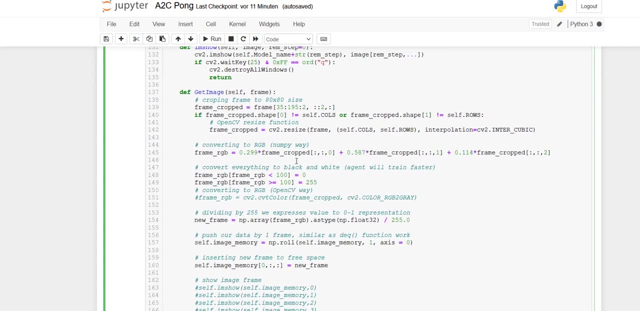 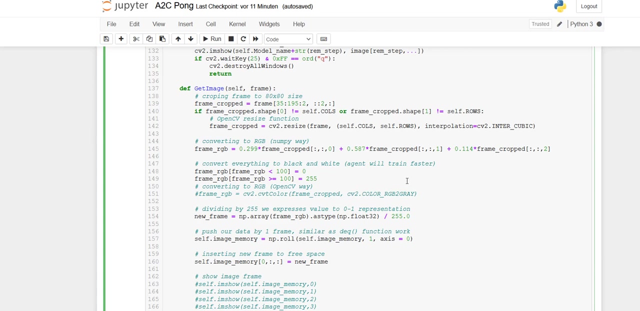 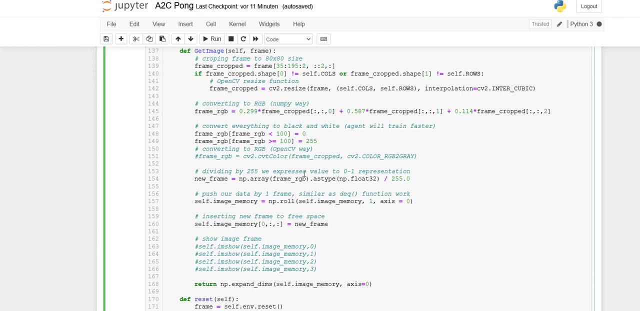 Model. You Can Also Use The Plot Method Here To Just Plot The Results Of The Model Afterwards. You Can Use The Method Here To Just 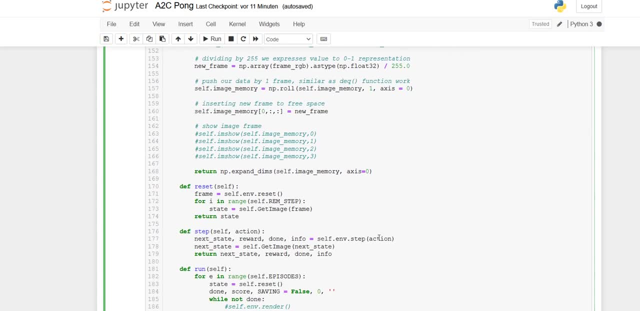 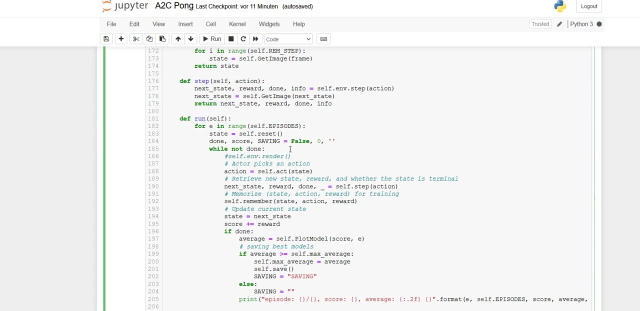 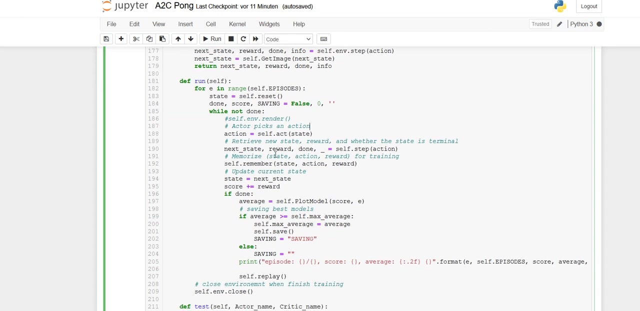 See The Results Right, How Your Agent Is Performing Against The Computer. You Can Just Visualize Everything In A Small Window, Then Updating The Action. 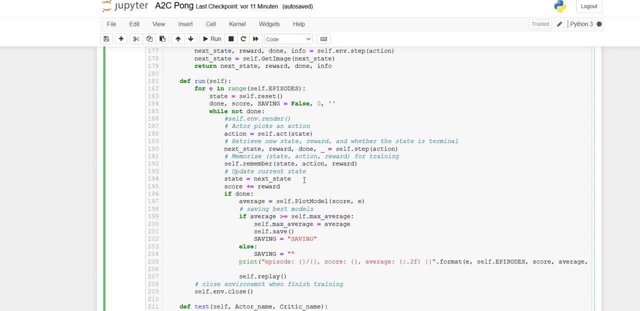 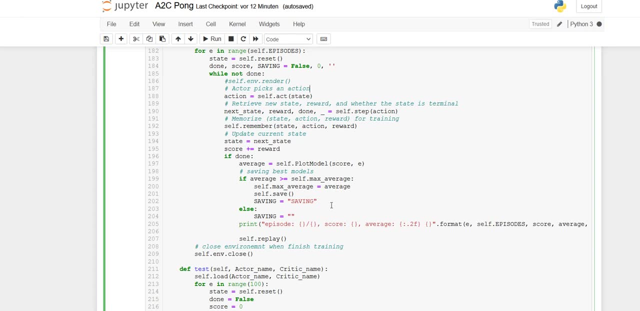 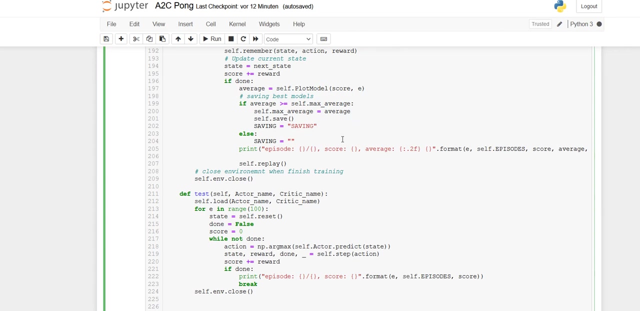 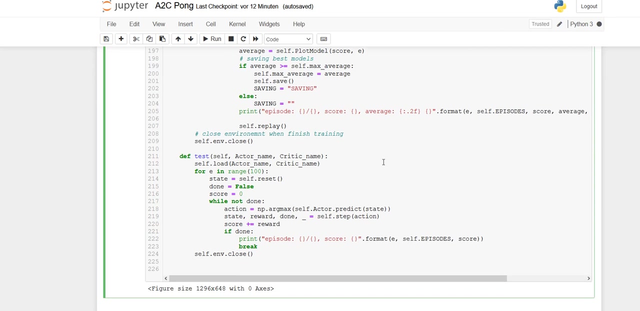 Then The Next State And The Reward And You Are Updating Everything And Afterwards You Going To Save Each Average Reward Here, And This Is Basically.